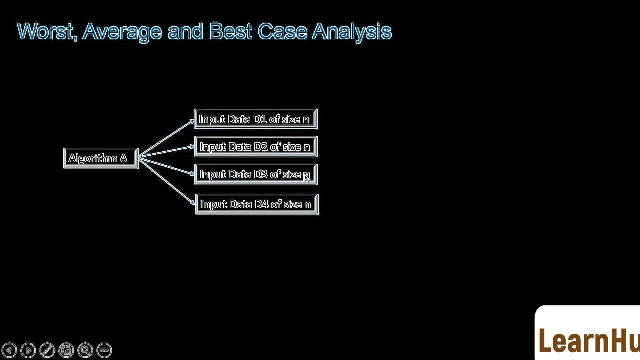 these are the different input data sets, which are all of size n. Now the running time taken in all these cases is different, So we can say that behavior of this algorithm depends upon the size of input as well as type of input. For analyzing these type of algorithms, we generally 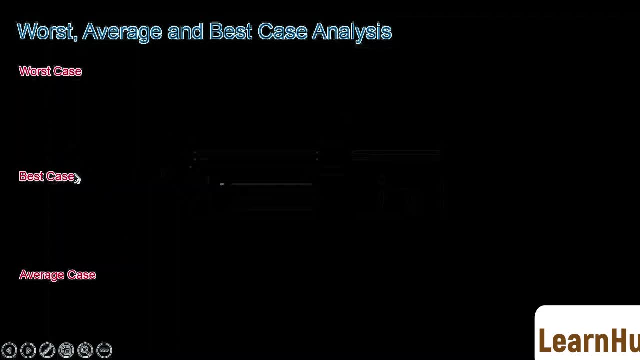 consider three cases: worst case, best case and average case. So we define the time complexity of the algorithm in these three cases. Worst case: time complexity gives us a measure of maximum running time that an algorithm will take for input size n. Best case: time complexity gives. 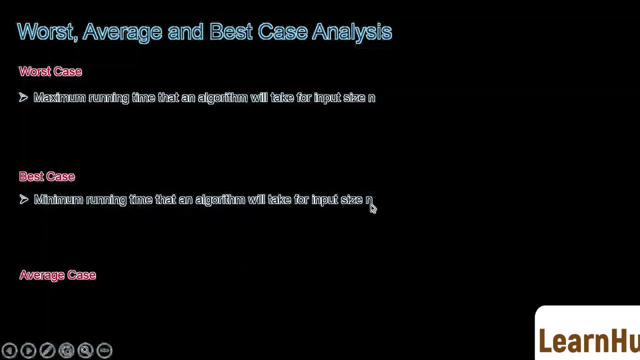 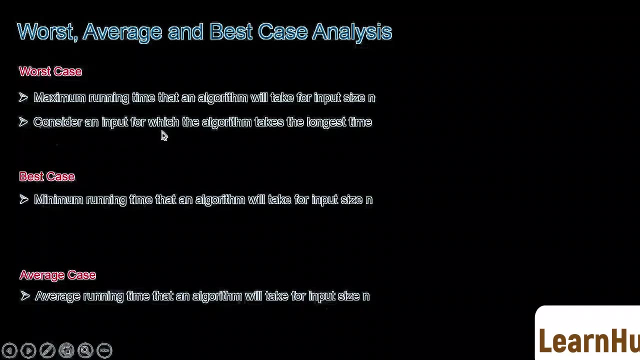 us a measure of minimum running time that an algorithm will take for input size n And average case time. complexity gives us a measure of average running time that an algorithm will take for input size n. In worst case, we consider an input for which the algorithm takes the longest time. 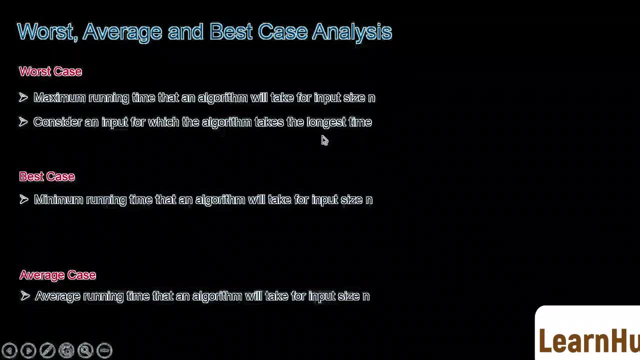 This input causes the maximum number of operations to be executed. For example, when we search for an element in an array using linear search, the worst case would be when the element to be searched is at the last place or is not present in the array. In that case, there would 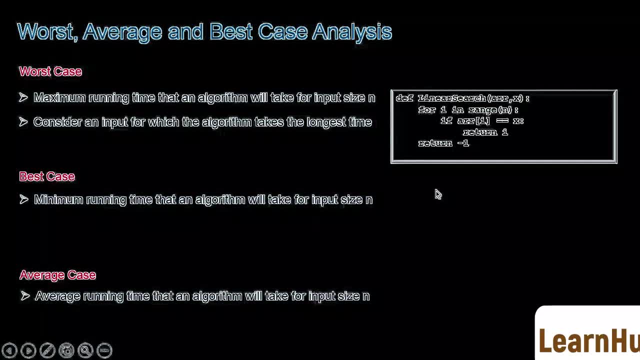 be n comparisons. So worst case time complexity gives us a measure of maximum running time that an algorithm will take for input size n And average case time complexity of linear search is order of n. In best case we consider an input for which the algorithm takes the 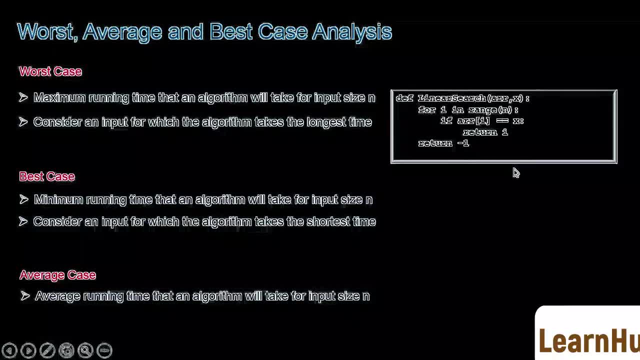 shortest time. So this input causes the minimum number of operations to be executed In linear search. the best case would be when the element to be searched is present at the first location of the array. In this case there would be only one comparison, So the best case time. 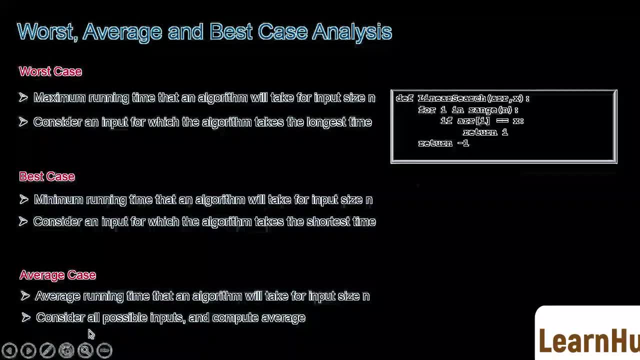 complexity of linear search is order of one In average case. we consider all possible inputs and compute an average. In this case we have to assume certain probabilistic distribution for the input data. The most common assumption is that all possible permutations of an input are equally likely.